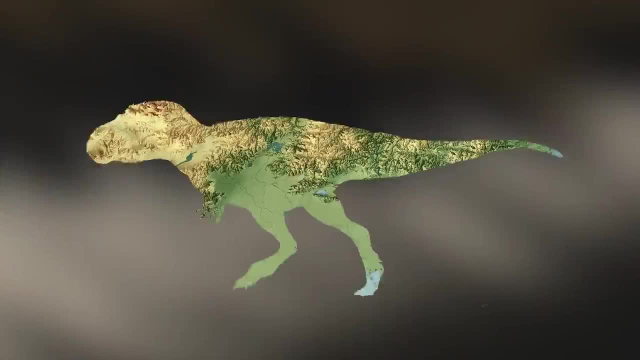 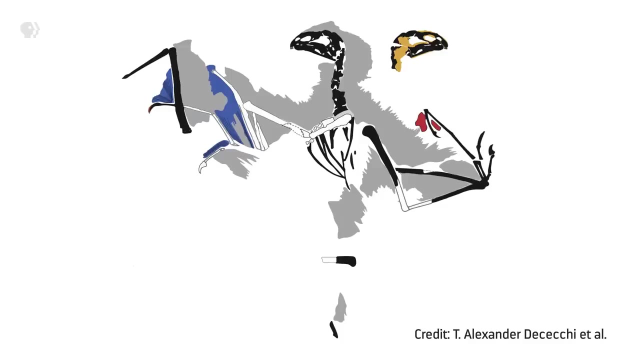 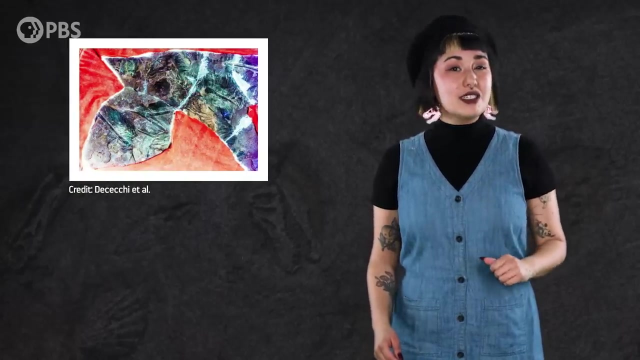 Thank you to Forreo for supporting PBS. In 2007,, in a quarry just outside a village in northeastern China, a farmer stumbled upon what seemed like some kind of small dinosaur fossil. A museum fought the fossil from him and in 2015,. 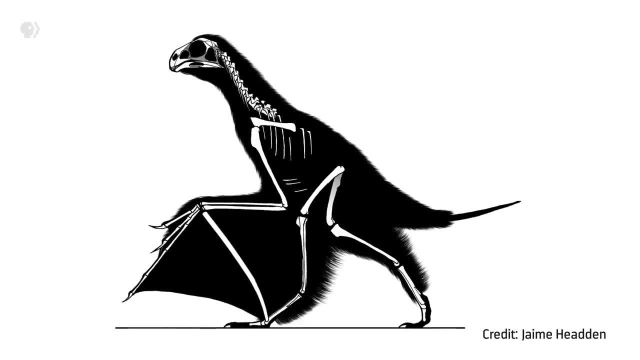 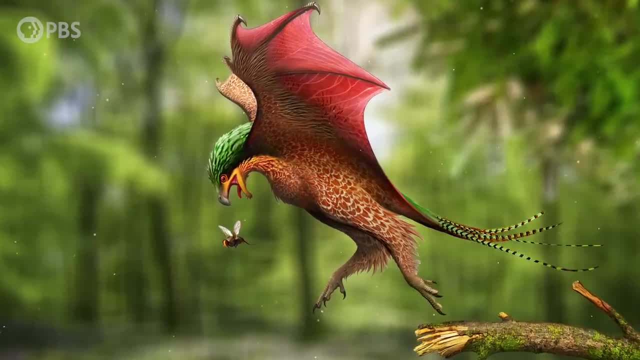 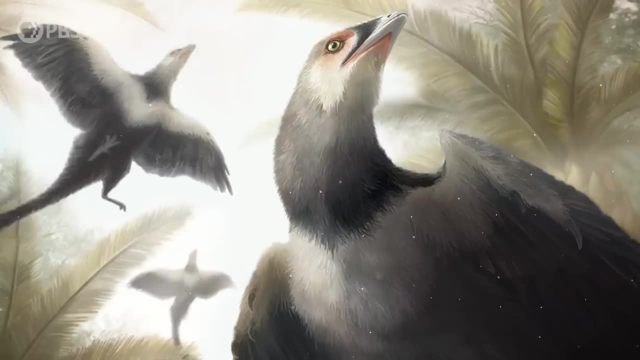 scientists announced that this chance discovery was a dinosaur unlike any found before. It was a pigeon-sized feathered creature from the late Jurassic period, Around 159 million years ago, And it seemed like a very close relative of the earliest birds, which also got their start around this time. 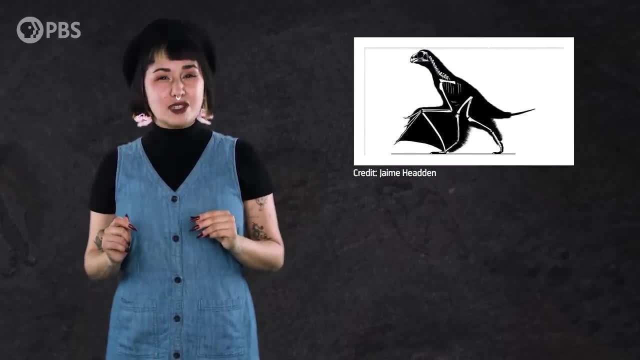 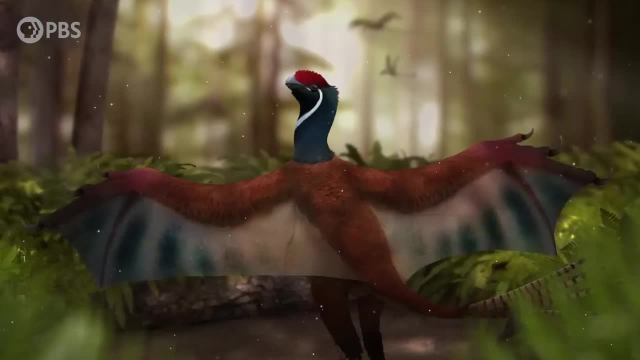 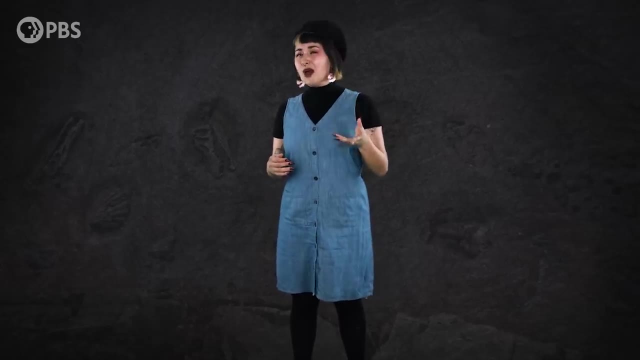 But it had one bizarre feature that had never been seen before in any ancient bird relative or in any other kind of dinosaur: Bat-like membraned wings. They named it ichi, which means strange wing in Mandarin. Overnight it showed us that there was a lot more going on near the origin of birds. 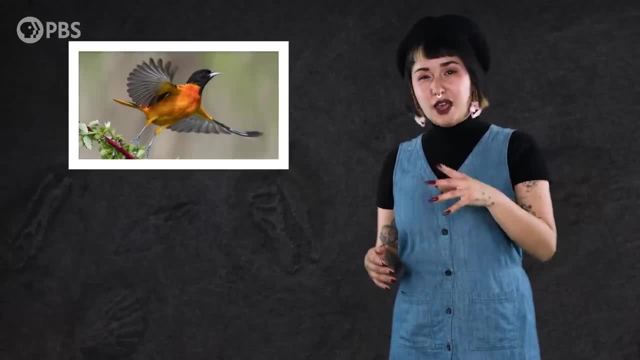 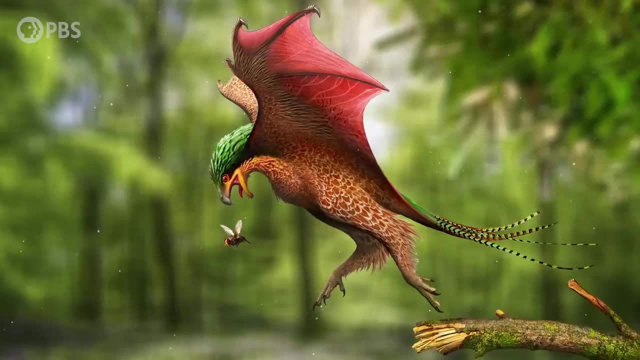 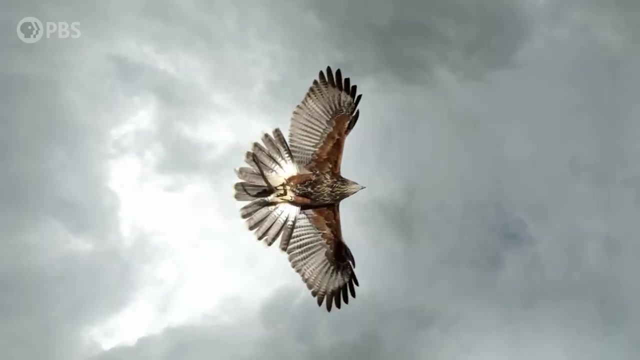 than we had predicted, And it's differences from birds actually makes the birds we know seem like the weird ones in comparison. Because if we take a step back, the discovery of ichi forces us to ask an important question From an evolutionary perspective: who really has the stranger wings? 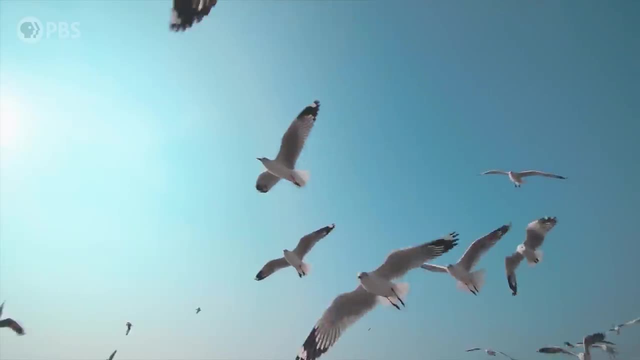 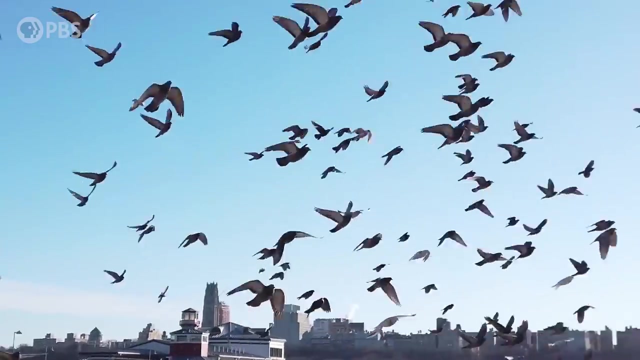 When we think of wings, many of us might picture feathers, Probably because birds are so familiar to us- We're just used to feathers- Feathered wings being the default for airborne dinosaurs And for decades. the fossil records seemed to back this up. 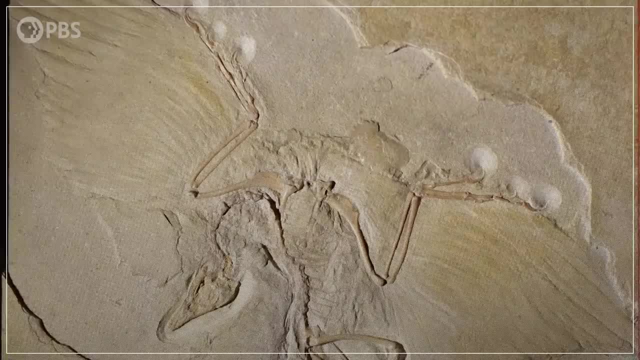 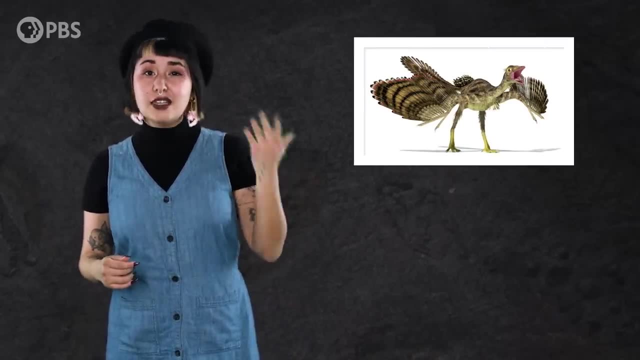 with paleontologists finding feathered dinosaurs in China and elsewhere, And though we knew we didn't have the full picture, the evolution of feathered wings and theropod dinosaurs, eventually leading to flight, was thought to have happened in a relatively linear process of gradual refinement. 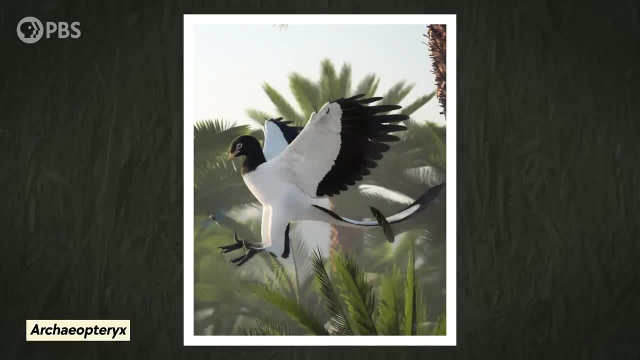 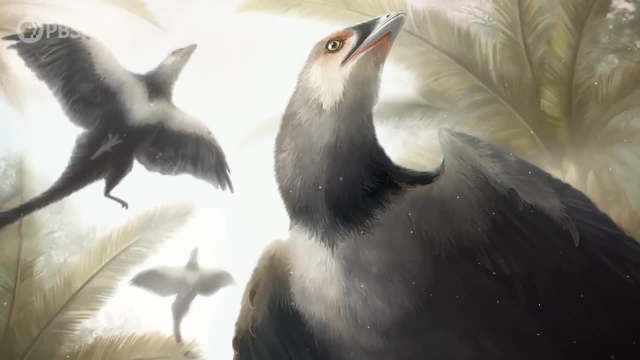 From poor fliers at first, like Angiornis, to Archaeopteryx, which could flap its wings enough to fly in short bursts, to the birds that fill the skies today. And there was no evidence to suggest otherwise, No reason to think that other bird relatives might have taken an evolutionary detour. and developed totally different kinds of wings altogether, But in the early 2000s a couple of interesting members of one particular dinosaur family were described. The first- in 2002, was the sparrow-sized juvenile specimen of Scansoriopteryx. 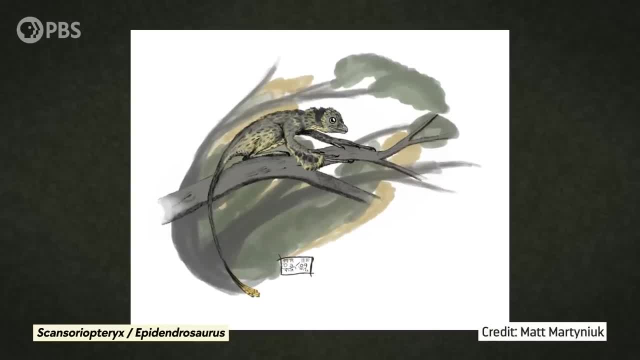 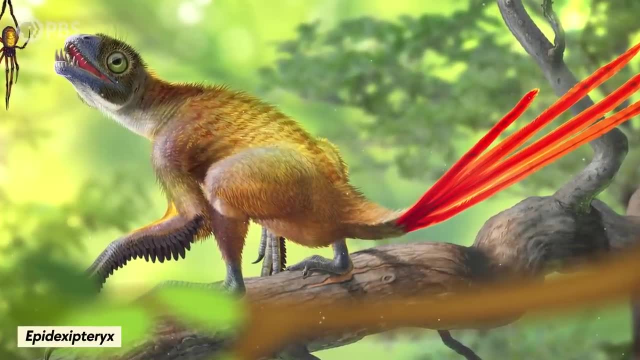 which is also called Epidendrosaurus, depending on which researchers you ask. It was followed by the magpie-sized Epidepsipteryx in 2008.. And based on some of the unique skeletal traits of these two species, researchers hypothesized that this family, the Scansoriopterygids, 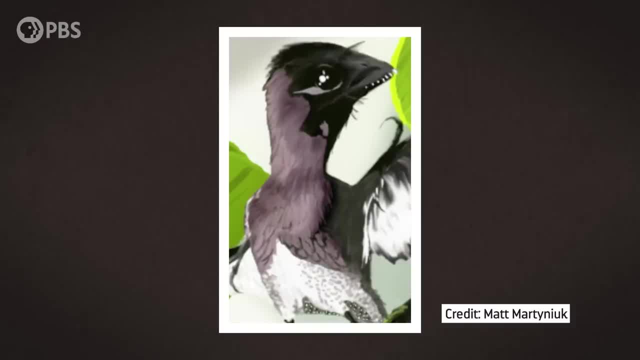 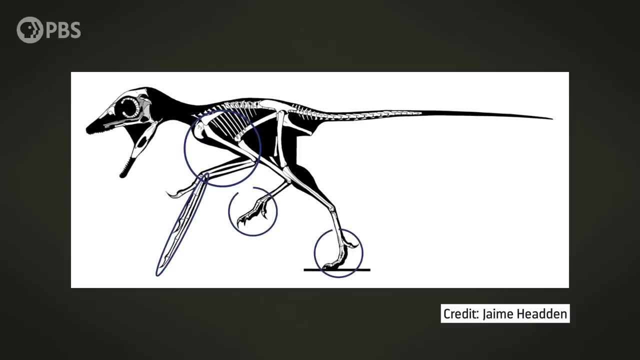 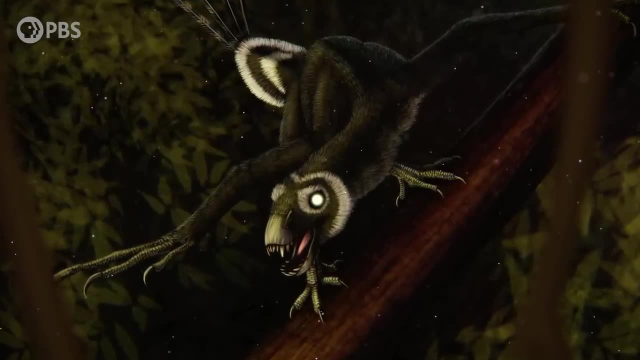 were small dinosaurs with an arboreal or tree-climbing lifestyle. These traits included their long arms, an extended digit on each hand and feet that seemed adapted for perching. So for over a decade, this family known only from a handful of other small fossils from the 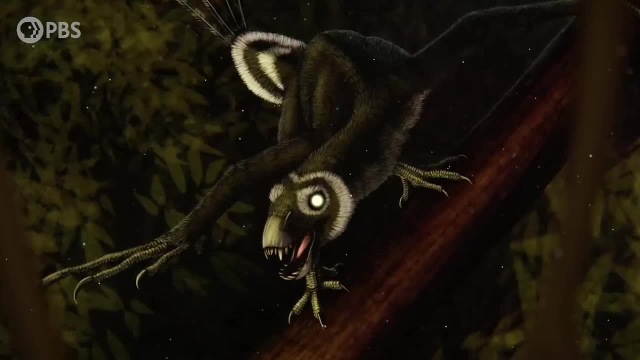 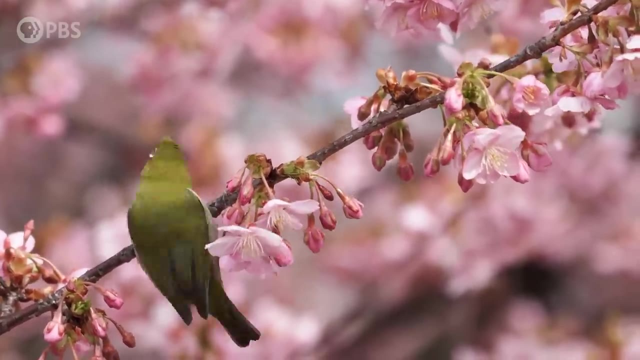 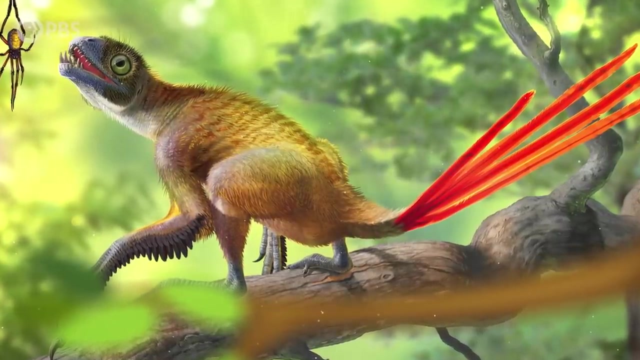 mid-to-late Jurassic period of China was just considered a strange group of dinosaurs, One that was closely related to the lineage that gave rise to birds and that had adapted to life in the trees. Now, this was already plenty fascinating. No other non-avian dinosaurs are thought to have been so arboreal. 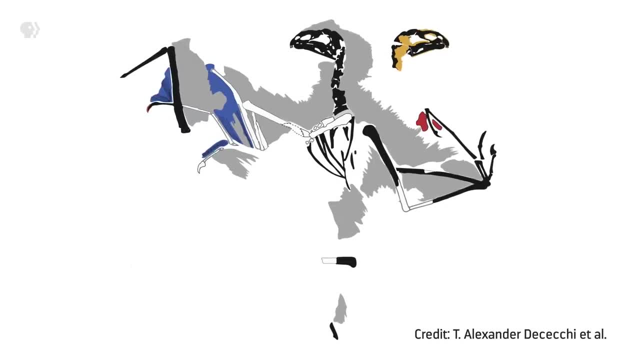 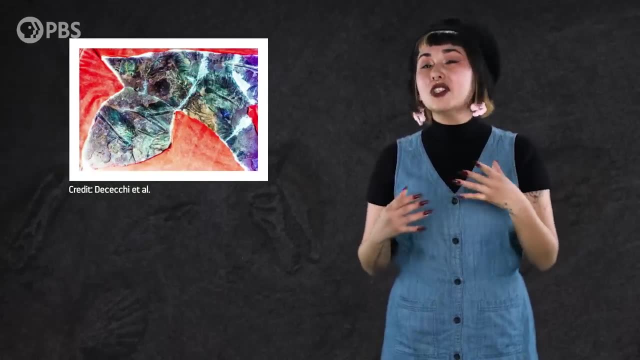 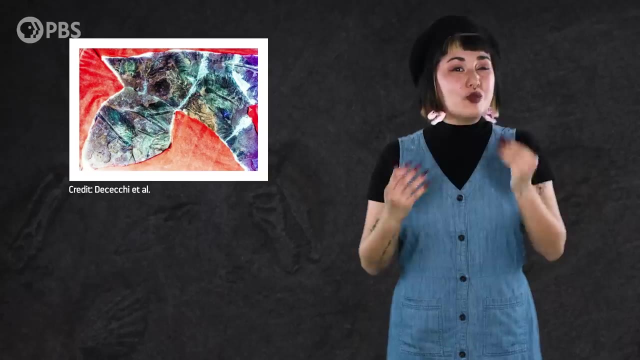 But the discovery of Ichi revealed that there was even more to this group than we originally thought. The incredible level of preservation of this specimen meant that some soft tissue elements were still visible, including clear evidence of a membrane wing attached to a rod-like extended wrist bone. that gave it structural support. 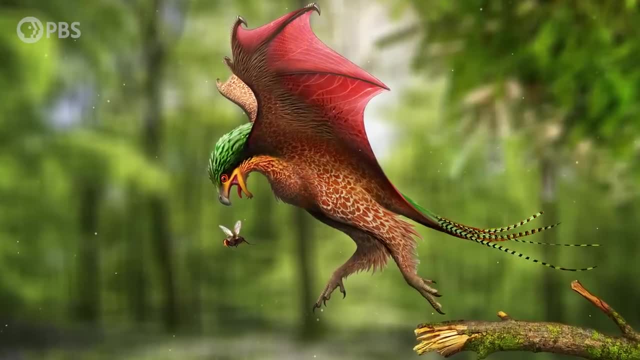 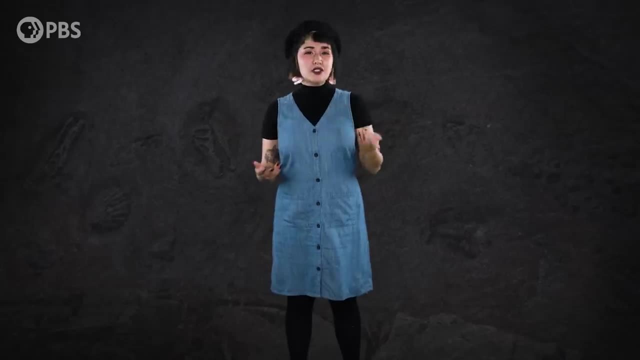 It suggested that Ichi and probably some of the other members of this family were not just climbing, but also taking to the air, And other Scansoriopterygids that were found later provided more evidence of this, Like Ambopteryx. 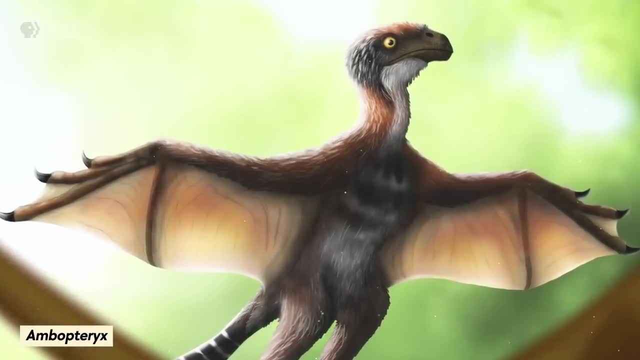 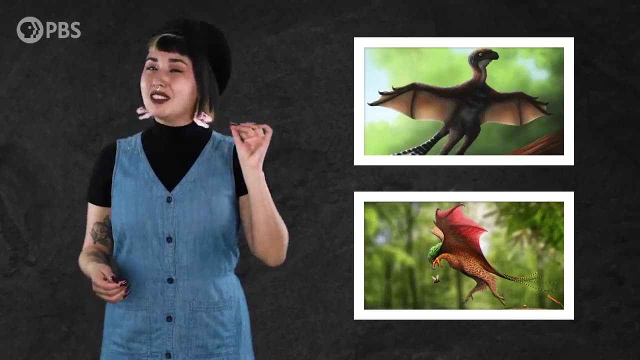 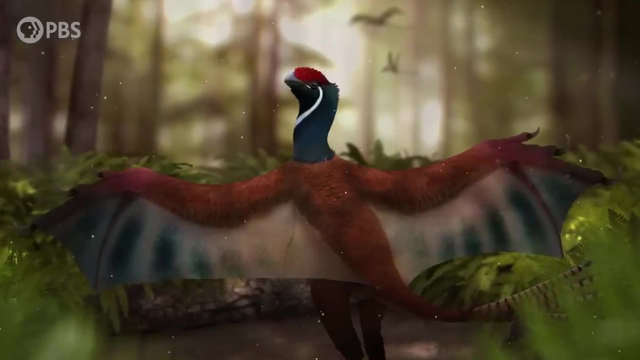 Which was also found by a farmer in northeastern China and described in 2019.. It's a close relative of Ichi that also has evidence of a membrane wing attached to the same extended wrist bone, So researchers propose that these dinosaurs represent a previously unknown. 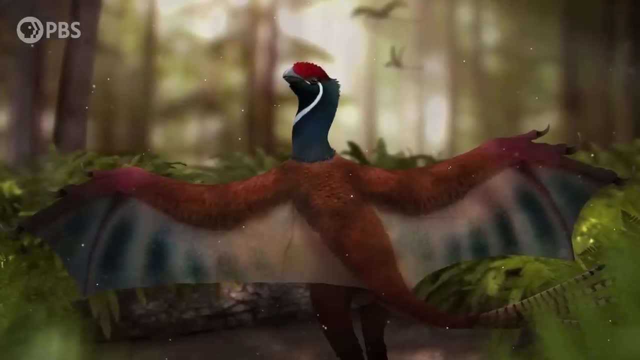 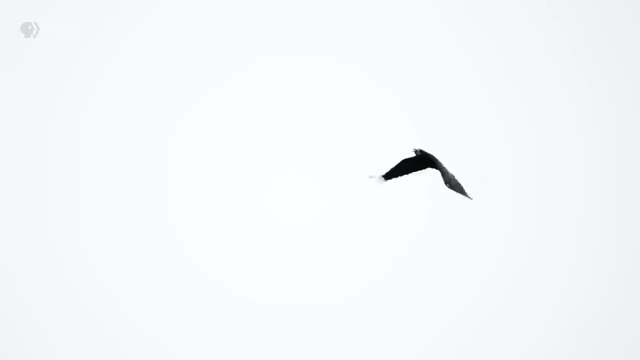 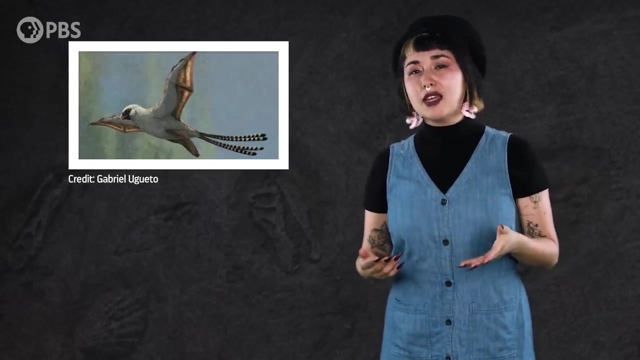 independent experiment in dinosaur flight, Maybe even one of many experiments near the origin of birds, The group that usually comes to mind when we think of winged flying dinosaurs, Though it's hard to tell from fossils alone whether they were capable of powered flight. like birds and bats, Or gliding flight like flying squirrels, Though gliding seems much more likely. One study from 2020 that modeled their flying abilities based on their wing structure even found that they probably couldn't do much more than very. 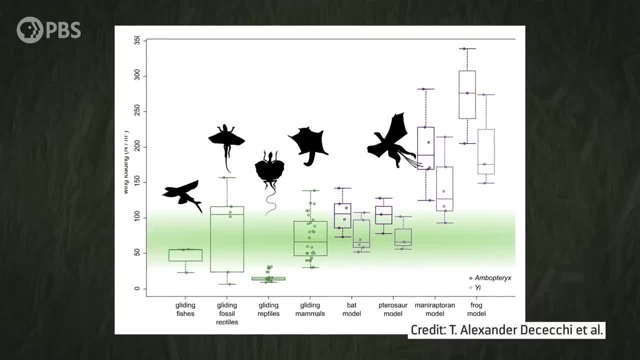 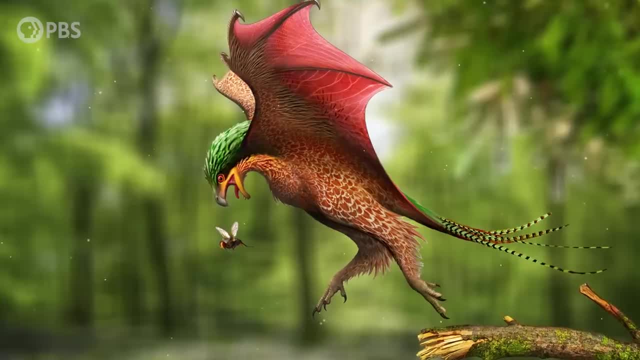 clumsy short-distance gliding between branches. They argued that Ichi Ambopteryx and the rest of their family were not just an experiment in dinosaur flight but a failed experiment, And that might be why all the species found to date are from. 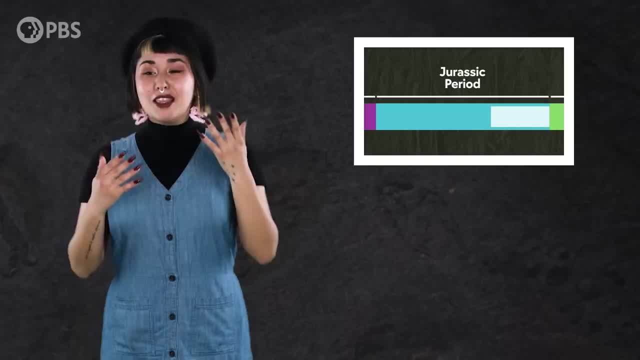 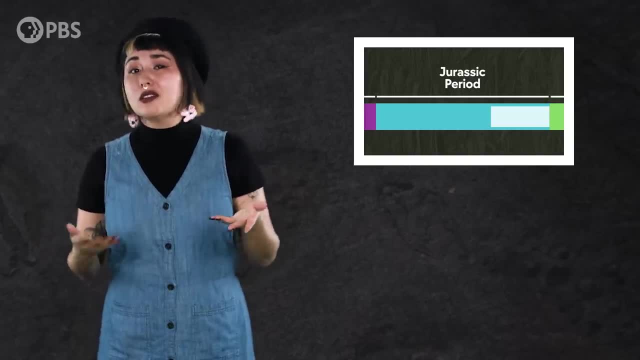 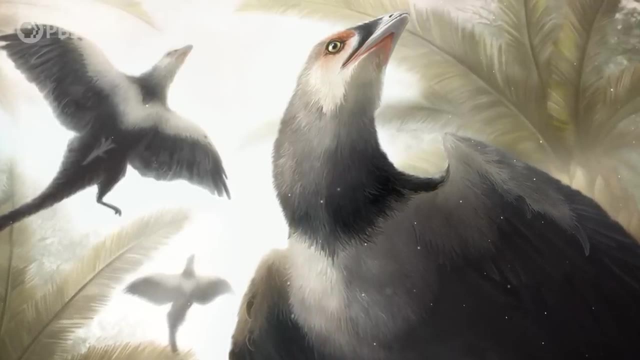 roughly the same time and place. in the late Jurassic The experiment hit a dead end due to competition with other groups like the ancestors and closest relatives of birds. It was in the late Jurassic, after all, that feathered wings also first appeared and gradually became more refined for flight over time. 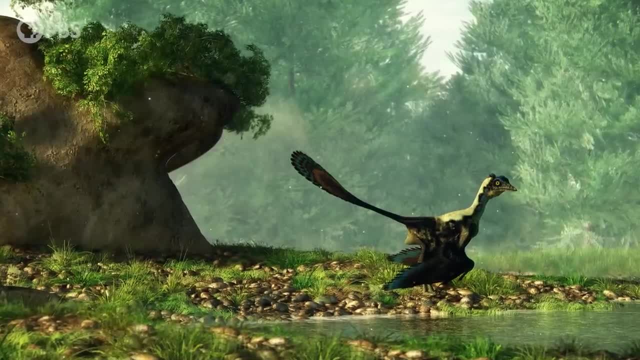 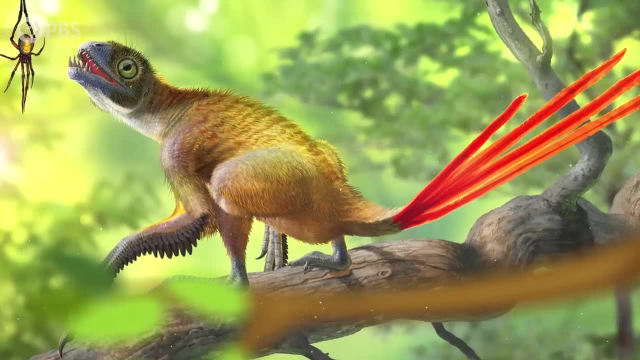 Eventually, this gave feather-winged dinosaurs flying skills that were much more impressive than anything the membrane-winged Ichi and its relatives had managed. Now, while the scansoriopterygids had both feathers and wings, they didn't have feathered wings. 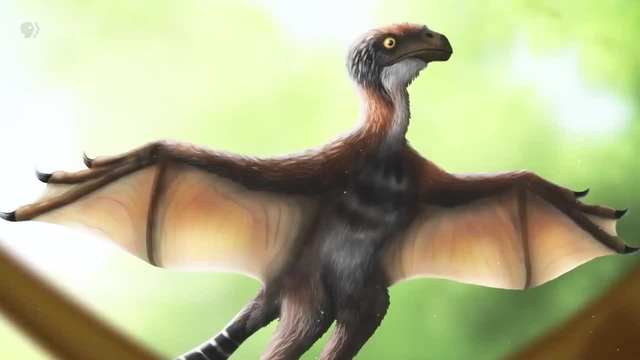 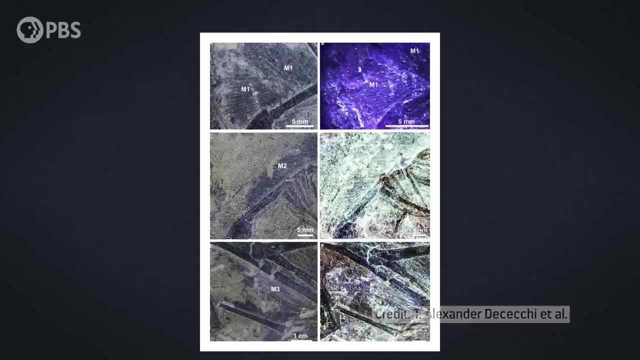 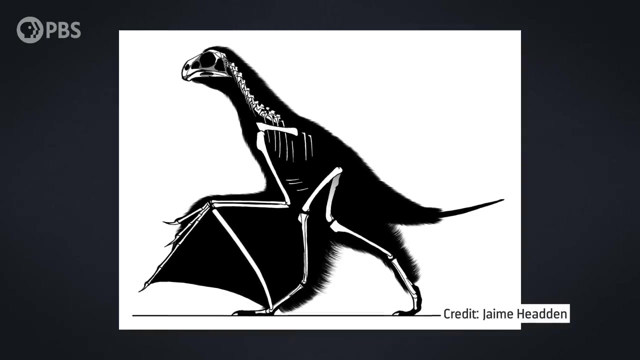 And they certainly didn't have the best of both worlds when it came to flight, Because their feathers, preserved in some specimens like Ichi, were simple, stiff and paintbrush-like. They were probably used for thermal insulation and for display, as they were in many other non-avian dinosaurs. 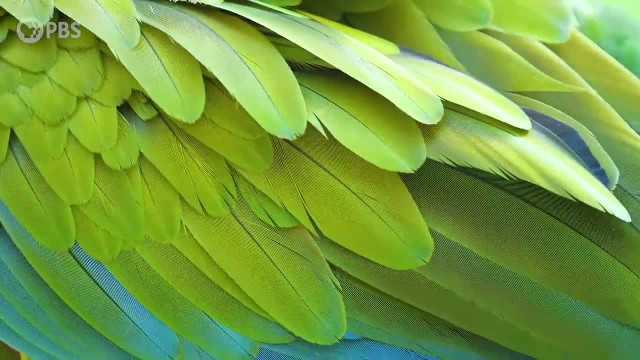 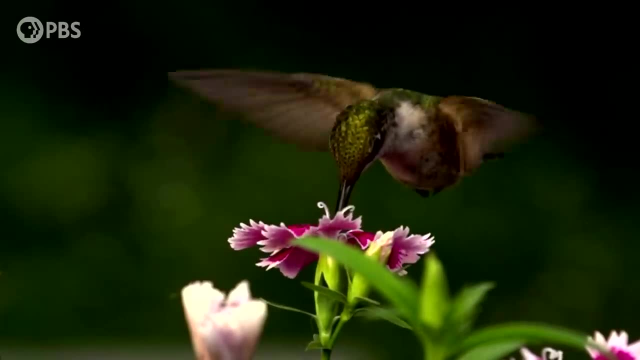 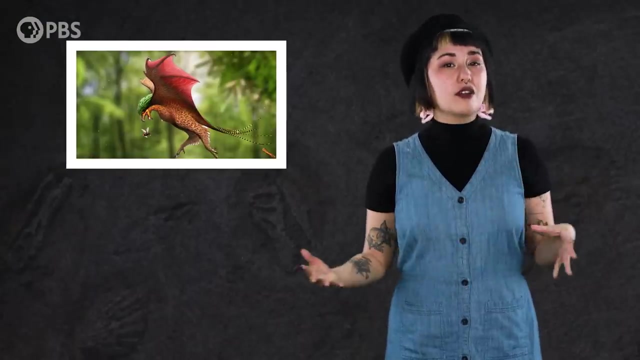 In contrast, the flight feathers of birds that cover their wings have a totally different and more complex structure. And because feathered wings are so successful today, we take them for granted and think of membrane-winged dinosaurs as strange and unusual. But if we take a broader view, maybe the way we think about Ichi and its relatives is totally backwards. 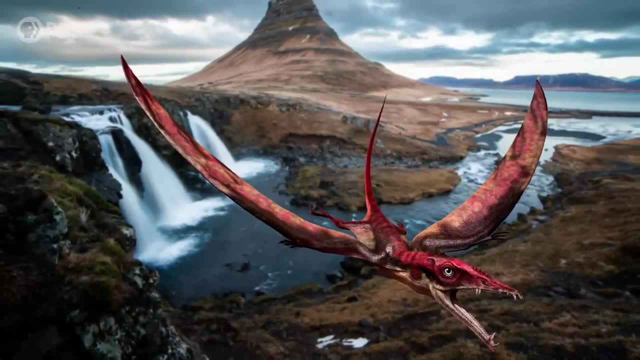 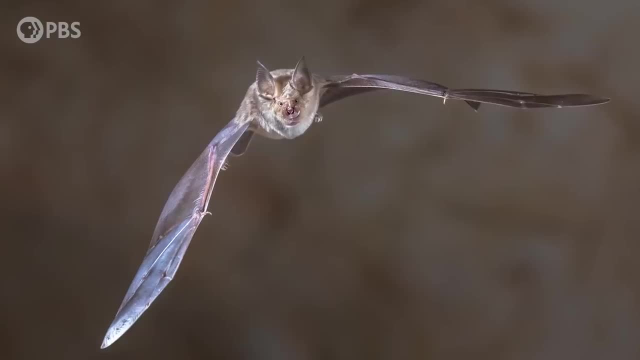 Membraned wings aren't strange at all, really. They've convergently evolved many times across the animal kingdom, From pterosaurs- the sister group of dinosaurs, to mammals like bats and flying squirrels. They show up so often for a simple reason too. Their simplicity. Membraned wings don't require nearly as much evolutionary innovation. The right mutations come together for an area of skin to grow more than usual and for the arms to change to support it. and boom, you've got yourself a membrane wing. 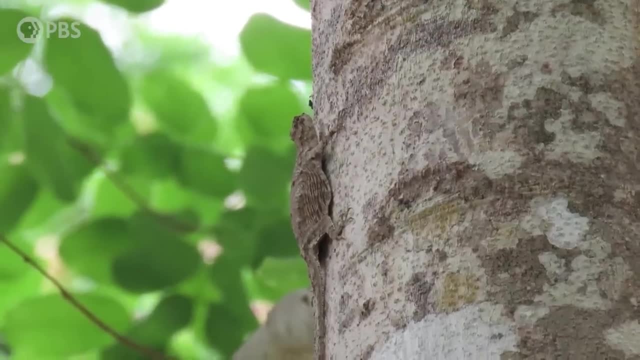 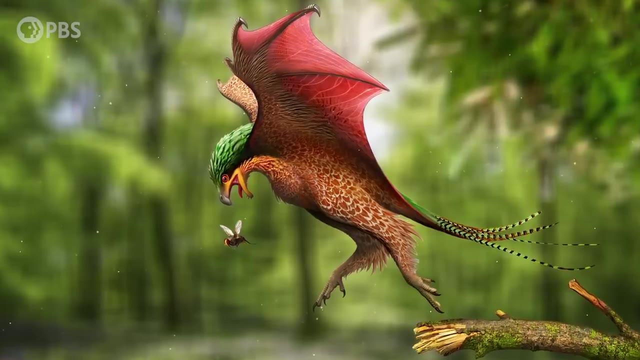 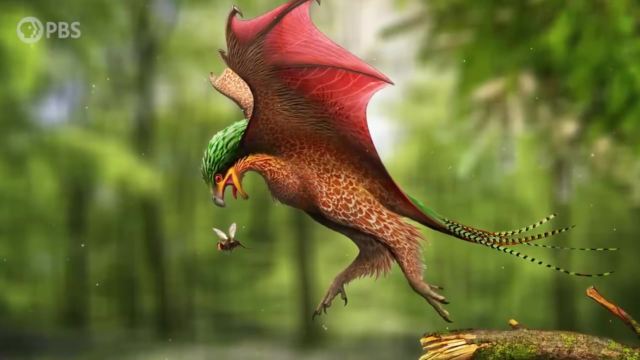 And these membranes often enable gliding And, in some cases, even powered flight to quickly evolve in previously flightless groups. So is it really surprising that some dinos, like so many others, went in this direction too, experimenting with gliding flight via a membrane wing. The fact that we saw them as strange is more like a testament to the success of feathered wings instead. But birds are not normal folks. Flight feathers are just about the weirdest and most complex things to ever sprout from vertebrate skin. 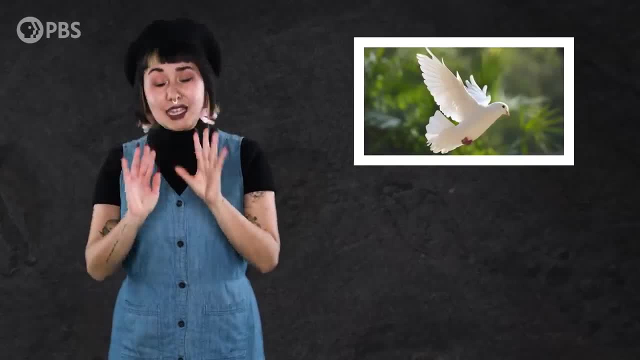 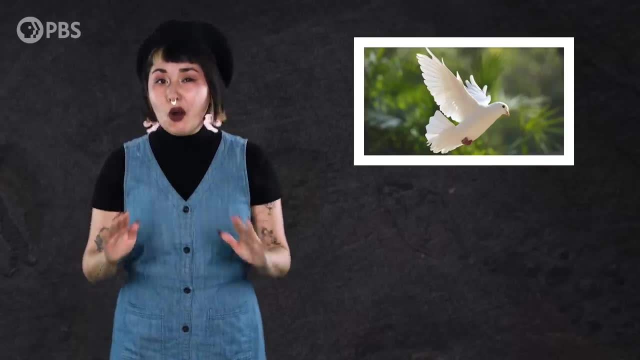 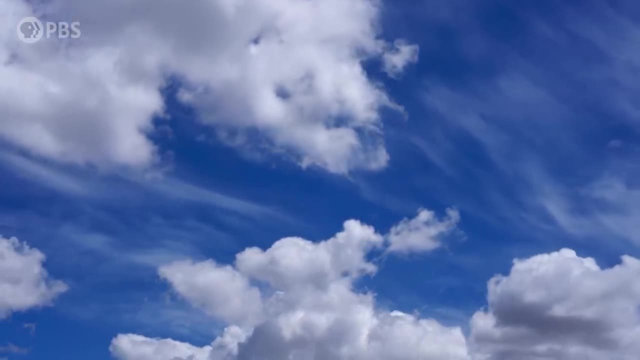 And, as far as we know, in the entire history of life on Earth, using feathered wings as a means of flight evolved only in birds and their closest dinosaur relatives. And if birds were to go extinct, the skies of planet Earth would be feather-free. 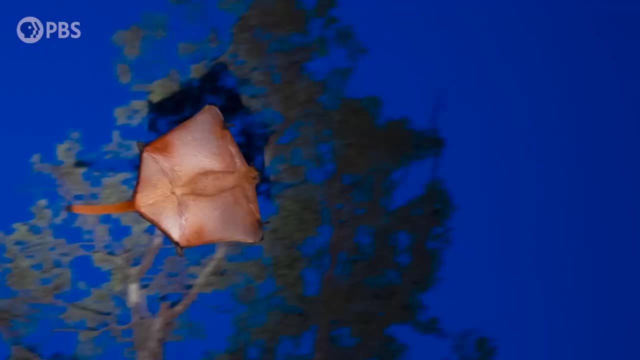 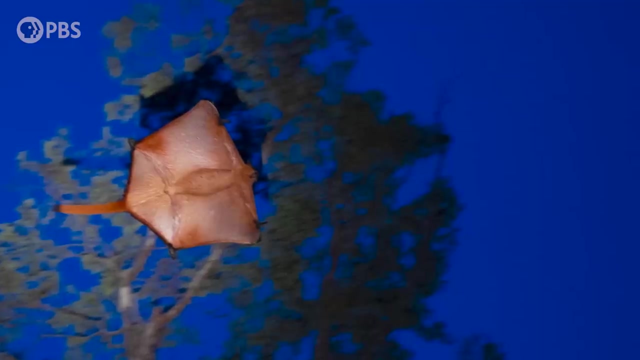 and might remain that way forever. But if every animal with a membrane wing went extinct today, on the other hand, you can comfortably bet that very similar structures would show up again before too long. They just don't require nearly as much evolutionary innovation. 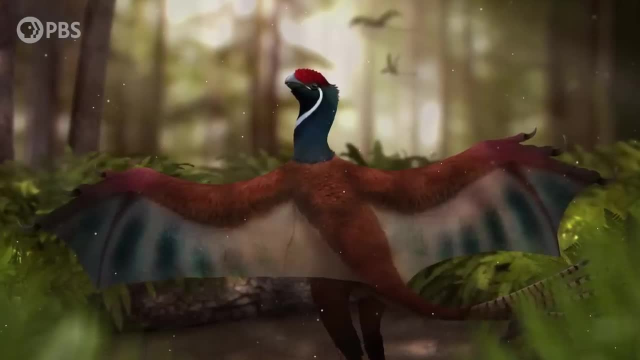 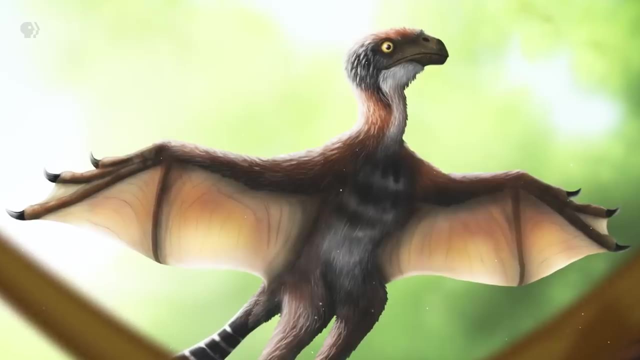 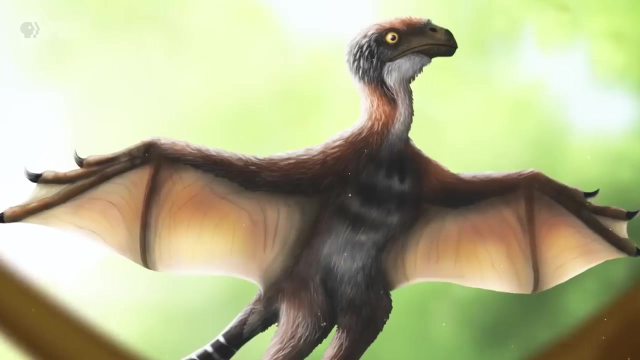 So, from a certain point of view, Ichi, our so-called strange wing, and the other scansoriopterygids weren't so strange after all, They were just one of the many diverse groups that independently experimented with this same simple approach to becoming at least kind of airborne. 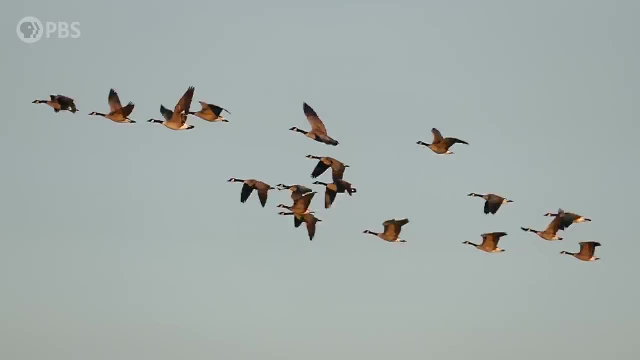 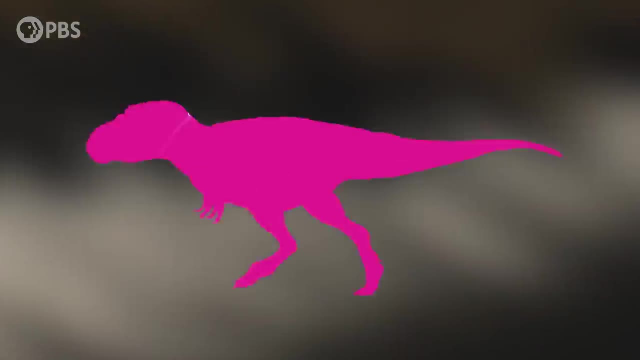 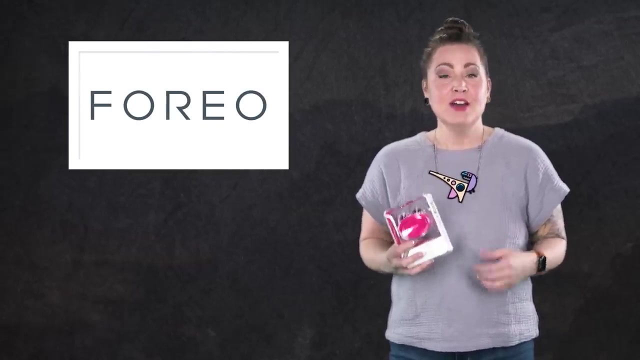 The unique feathered wings of birds instead are actually the strangest wings of all. Thank you to Foreo for supporting PBS. Among many inventions that define the world around us are those within the well-being industry. Foreo Sweden is a brand in the space where the beauty and tech worlds meet. 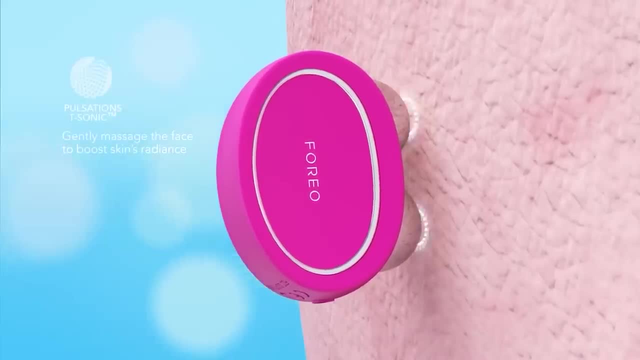 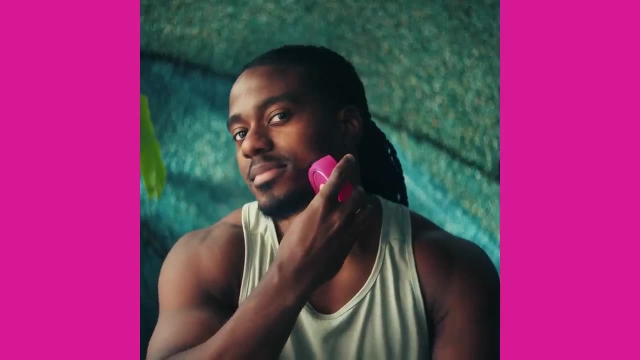 Their skincare devices use T-Sonic pulsations which travel through the outer layers of the skin to channel a low-frequency massage to help relax facial and neck muscle tension points and improve blood flow. And Foreo microcurrent technology with its low-voltage electrical current. 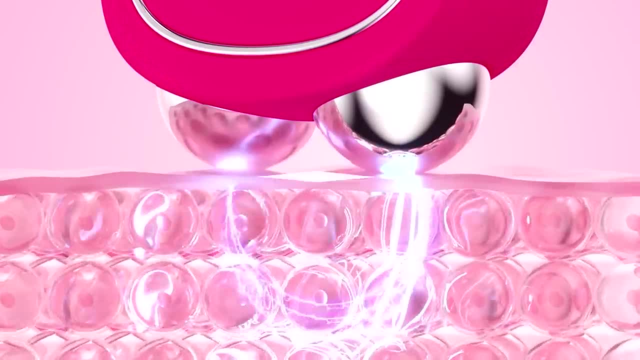 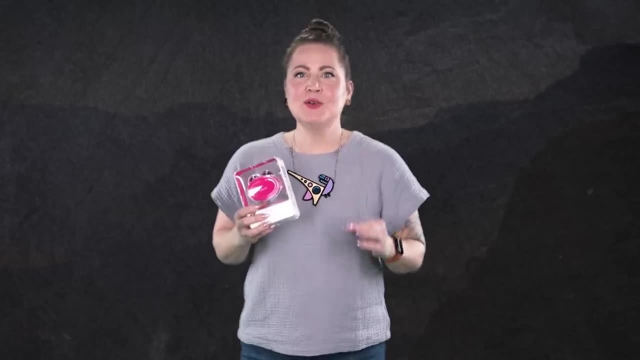 offers a natural, non-invasive and instant facelift. It helps to contour and lift the skin and facial muscles. The Bear by Foreo is the world's first FDA-cleared medical microcurrent device with an anti-shock system designed to visibly improve signs of aging by 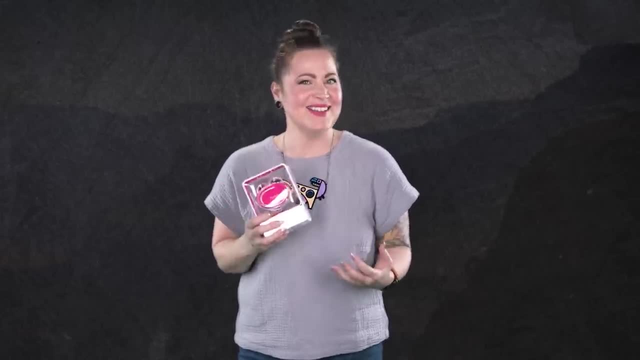 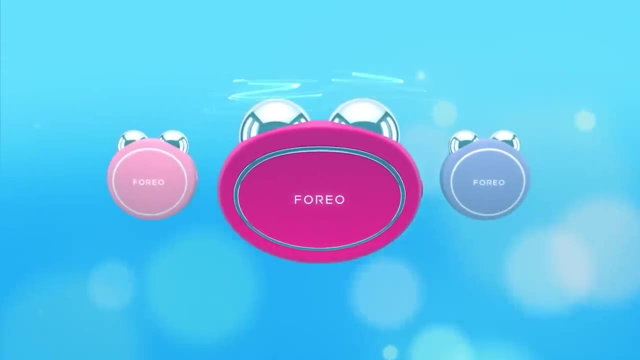 energizing and firming the dozens of muscles in the face and neck. If you're looking for a present for an anniversary, a birthday or any other special occasion, The Bear by Foreo is available- Available online or in stores. Thanks to the FOLLOWING EONtologists for their support. this one 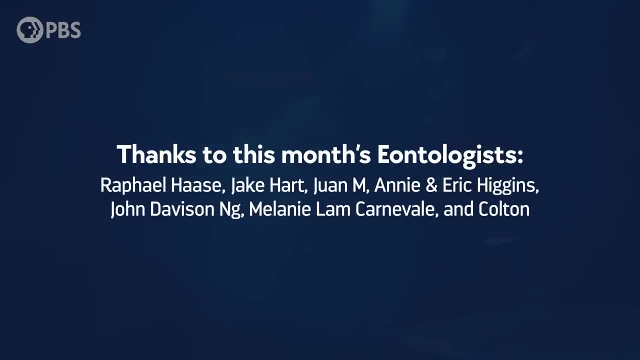 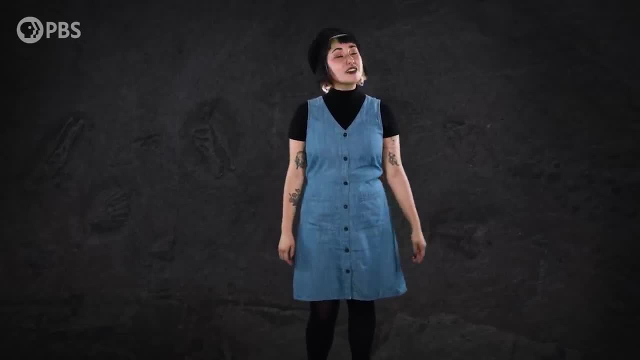 Raphael Haas, Jake Hart, Juan M, Annie and Eric Higgins, John Davidson Ng, Melanie Lamb-Carnivale and Colton. By becoming an Eonite at patreoncom slash eons- you can get fun perks like submitting a joke for me to read.